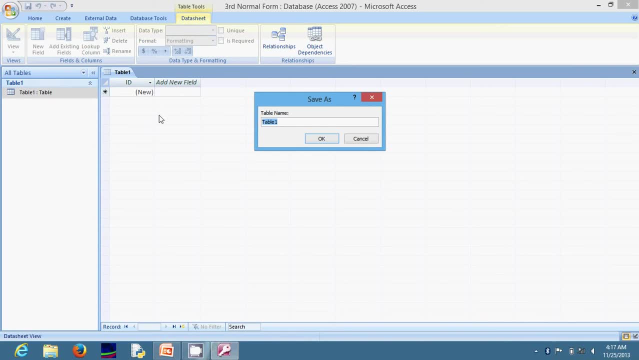 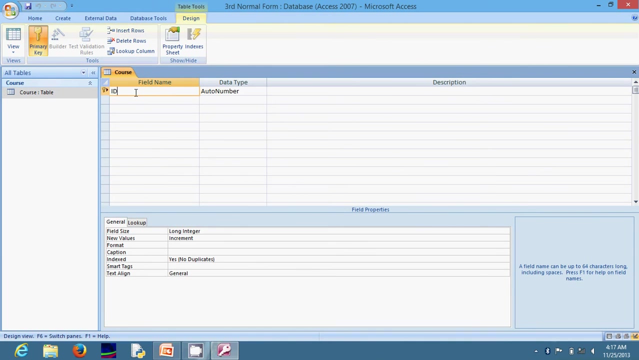 So we're going to have First, let's go to design view. I'm going to call this first table table course, Table course. So okay, For the design view I'm going to. I have course code. 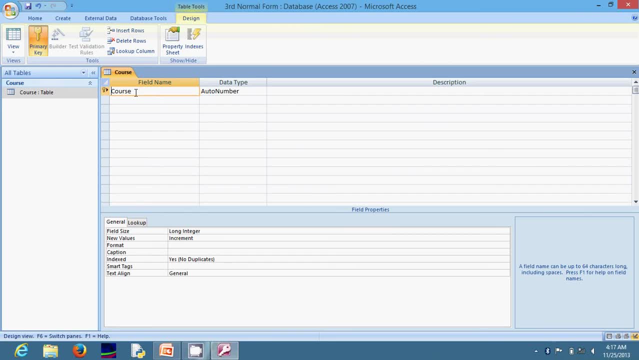 I'm sorry The ID will not be there And I have course code For this auto number. of course it will be tests And this will be 7.. Then I'm going to have course name. Of course tests. 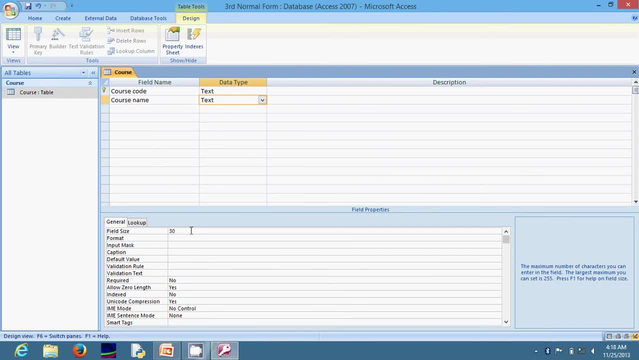 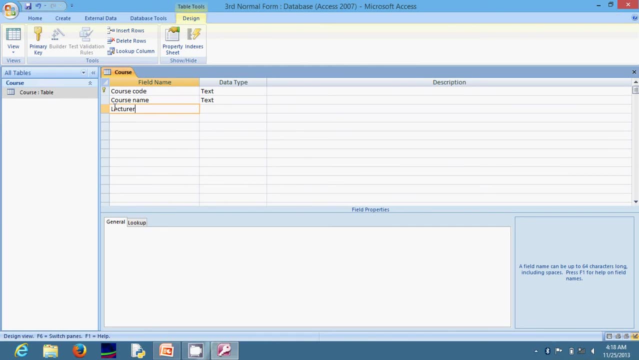 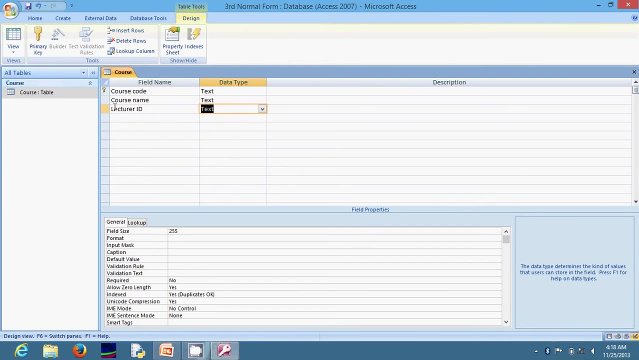 And this will be 13.. And lastly, I'm going to retain lecturer's ID. What I'll do is I'll take only lecturer name away from this table, And that's a better idea, So I'll retain lecturer ID. 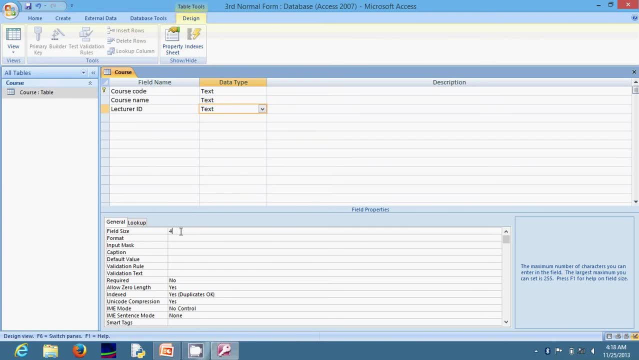 So tests Then 4.. Alright, If you like, you can write description here if you want, But of course the primary key will be the course code. Now, once you're done, you save this table. Save the table. 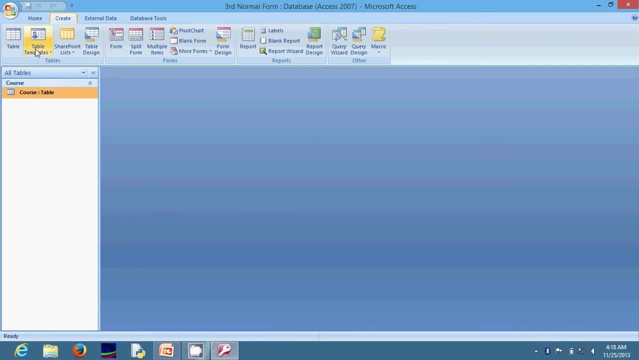 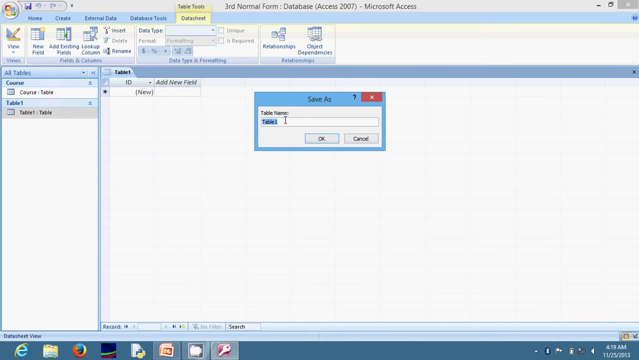 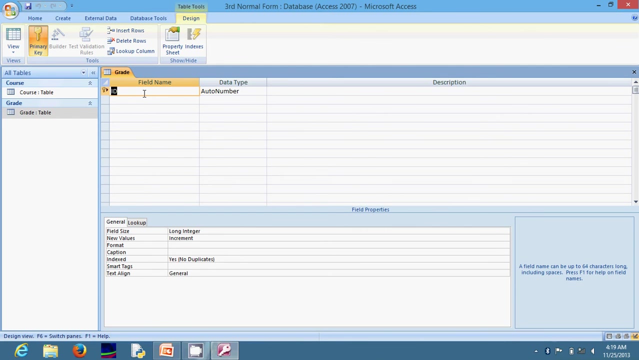 And exit. So we're going to create another table And we're going to call this one table grade Now for this table we're going to have. Of course, this is similar to what we already did in table 2 for the last lesson. 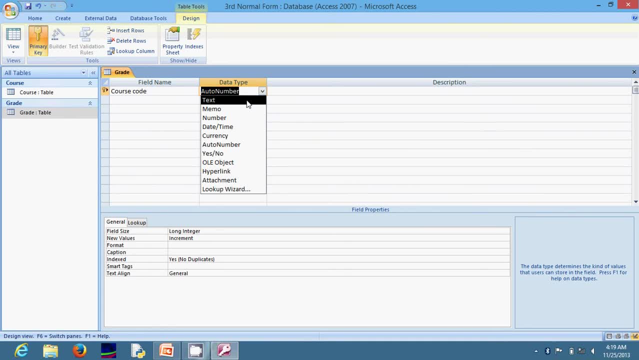 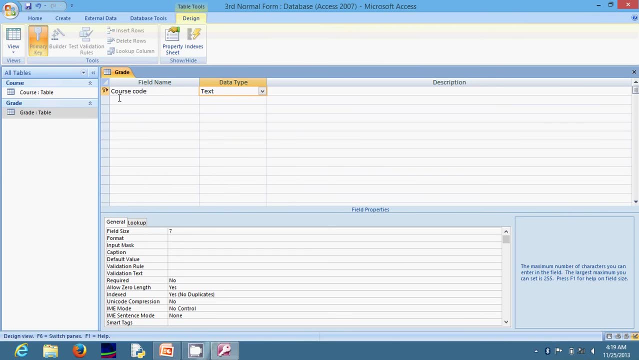 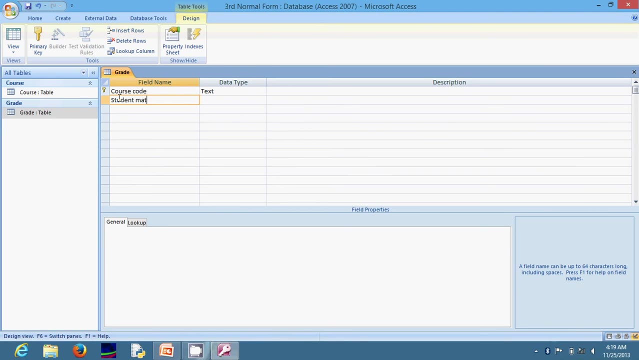 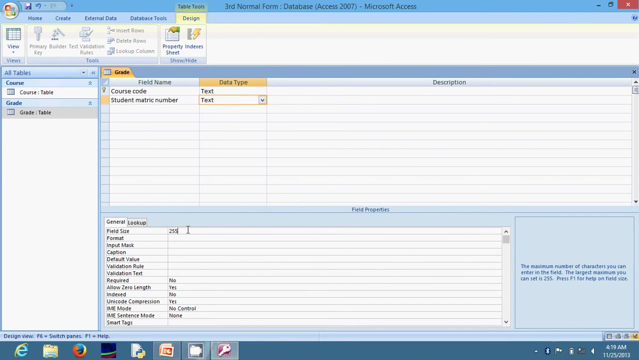 Course code. This will be tests And it's going to be 7.. Then I'm going to have student's matrix number And it's going to be test also, And I'm making this 5.. Don't forget it will also serve as a primary key. 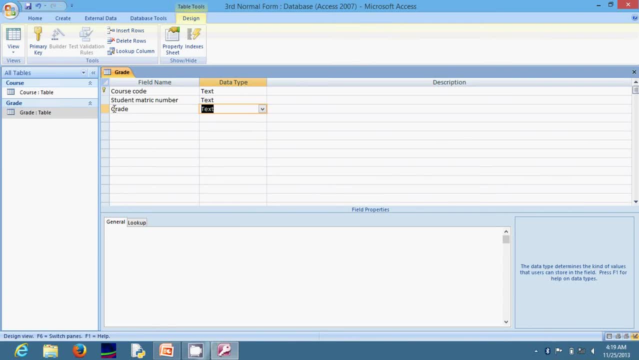 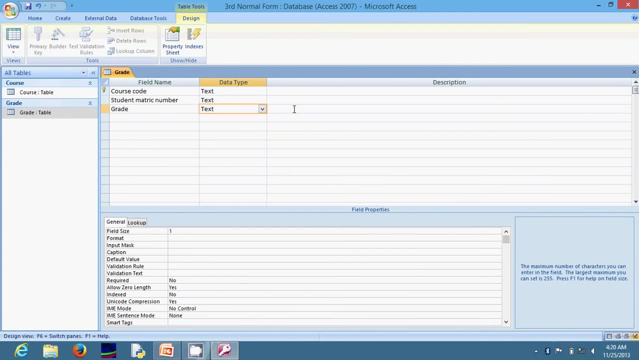 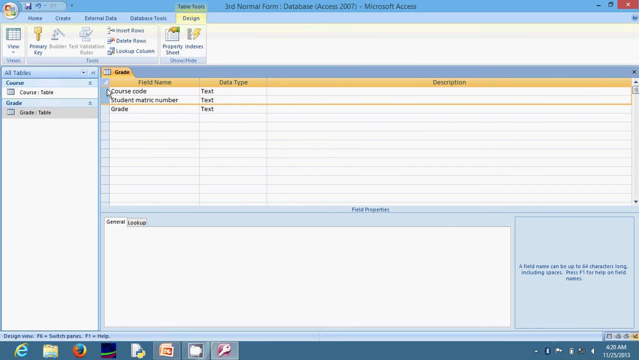 I'm coming. Then we'll have grade, which is test also, And grade will be 1.. Alright, Now, like I said, this will also serve as primary key, So I'm going to remove from here. I like this to using the shift button. 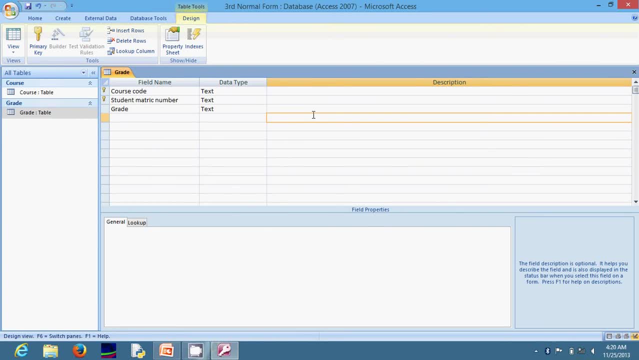 Then press this, So I have this. So here, course code and student's matrix number will serve as a composite primary key. One of them will be the primary key because grade needs both of them. Alright, So if you like, you put description. 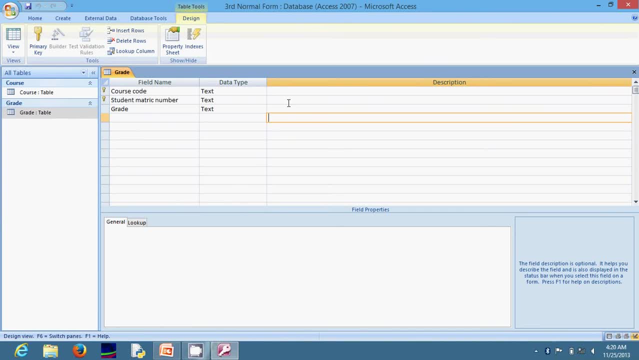 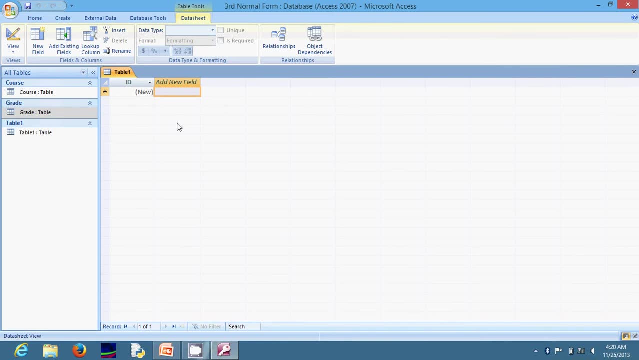 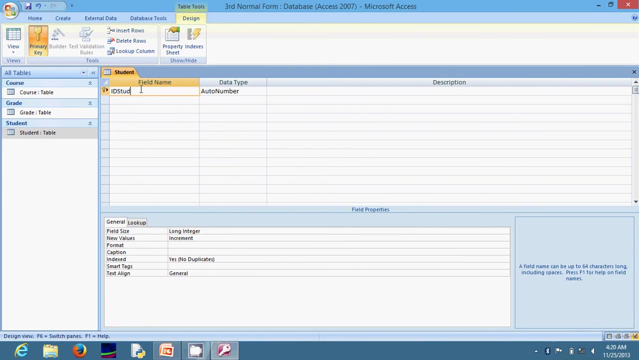 If not save And exit, Then we're going to create another table And I'm going to call this table grade Table: students, Students. So okay, For students, we're going to have student's matrix number. Of course, that will be the primary key for this. 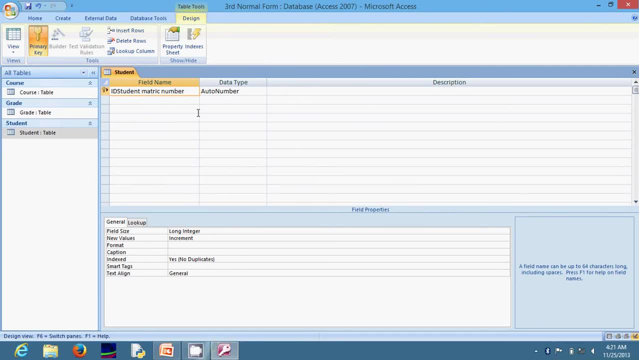 Matrix number And of course we're going to have this And it's going to be a test And we expect this to be 5. And of course, like I said, it's a primary key. Then we're going to have student's name. 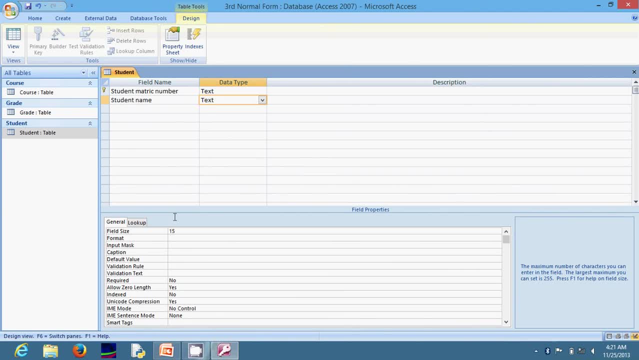 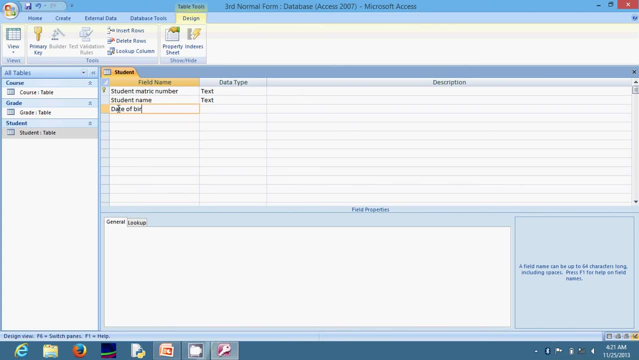 Which will be a test. We don't expect that to be more than 15 characters And we're going to have date of birth And this is going to be date stroke time And, of course, like I said, short date is preferable. 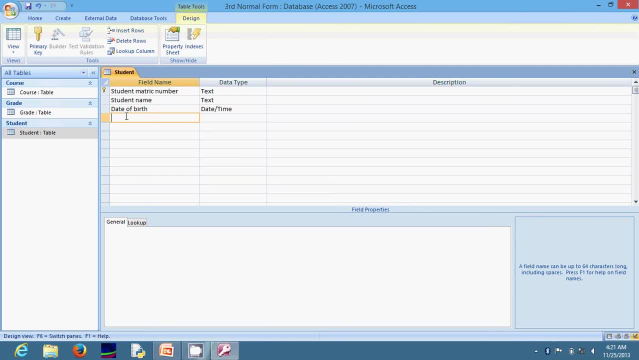 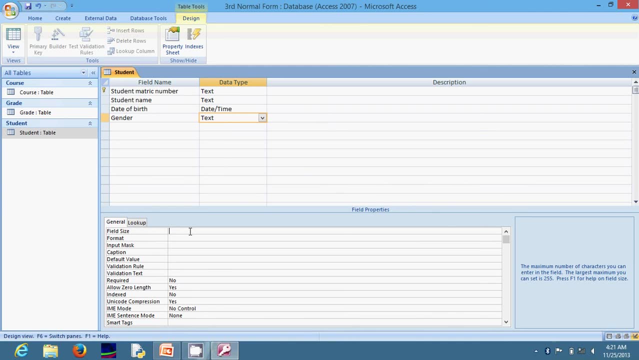 Then we're going to have gender as a last part And we'll be going for cis, because female is cis letters, And that'll be it. We want to describe your field. If not, ensure you save And you can close. 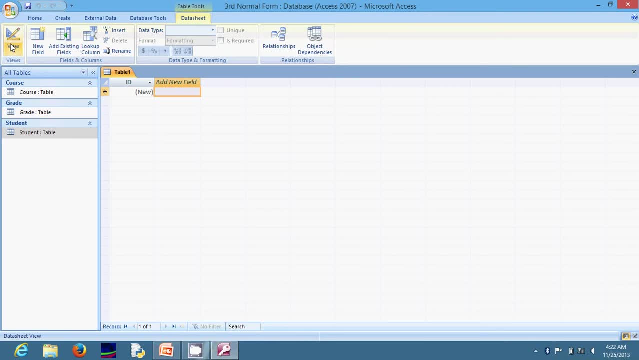 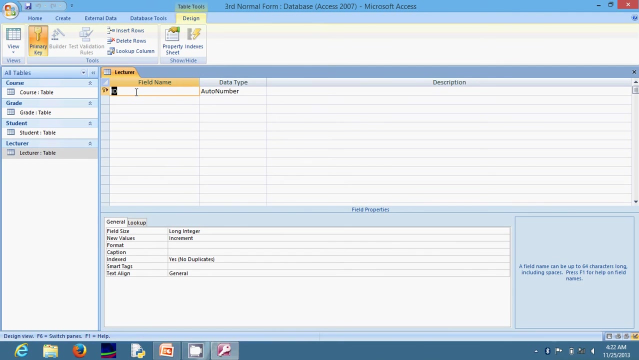 The last table we'll be having will be table lecturer, So let's quickly do that, So okay. So for this, now we're going to have the lecturer ID and the lecturer name, The two attributes causing issue with our last lesson. 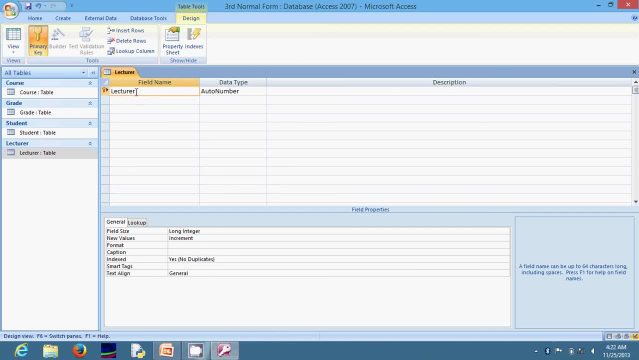 So we're going to have lecturer ID. Of course, this will be test too, And then I made this 4. It's a primary key And I'm going to have lecturer name. It will be test also, And this will be 15.. 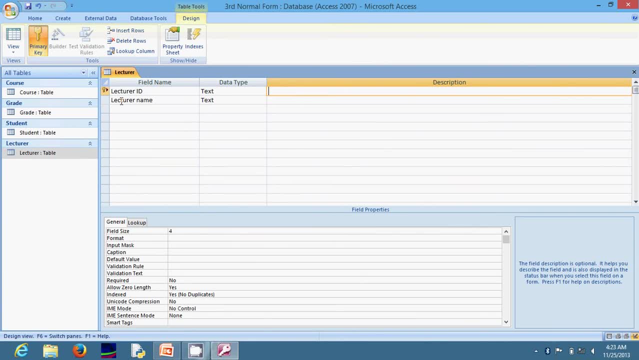 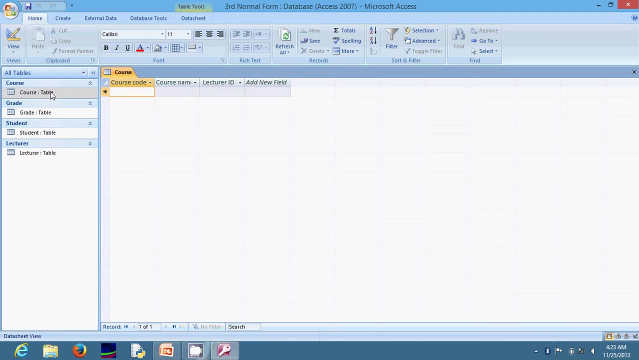 So you can describe if you want. So I'm going to save And I'm going to close this. So let's check what we have. Course code: That's course code, the course name and the lecturer ID. 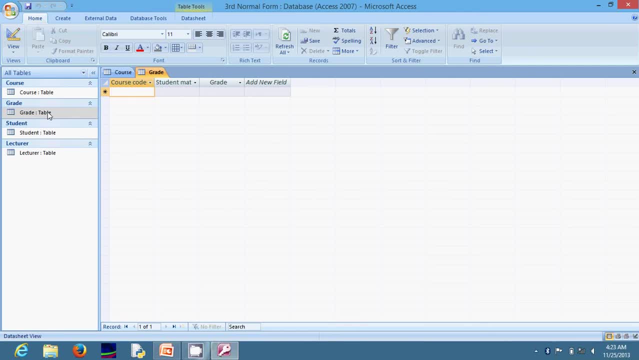 It's okay. Grade: That's your course code, Your student's matric number And the grade. That's okay too. Table students: We have student matric number. student's name, date of birth, gender- That's okay too. 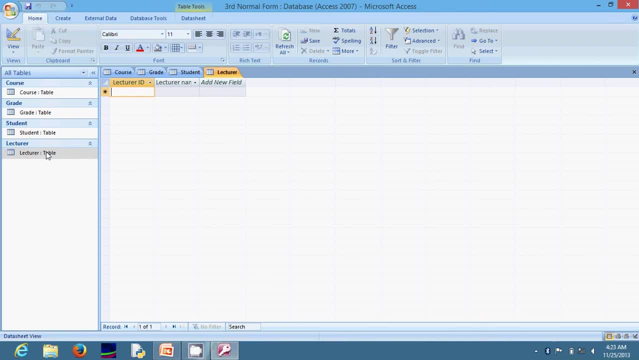 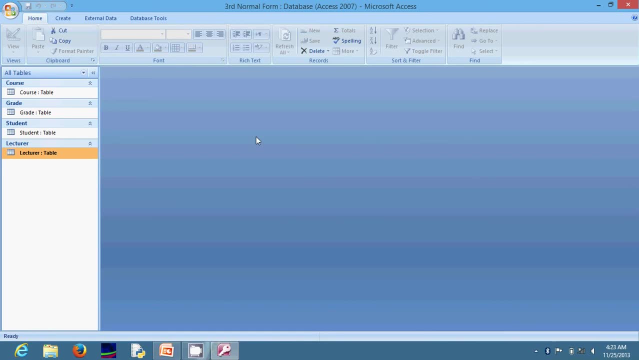 Then lecturer table. We have the lecturer ID and the lecturer name, Alright, So we can go ahead now and create the link. Don't forget that there's no link yet between these tables, So what we're going to do is we quickly create the link. 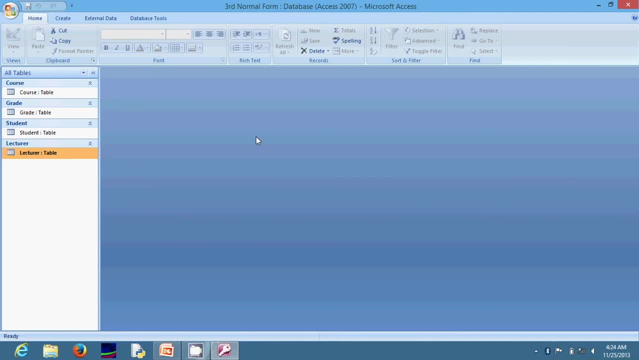 Now to do the lookup wizard. what we're going to do is we're going to link course code in table course to course code in table grade. So that means table grade will be my target. So what I'm going to do is from table course. now I'll go to design view. 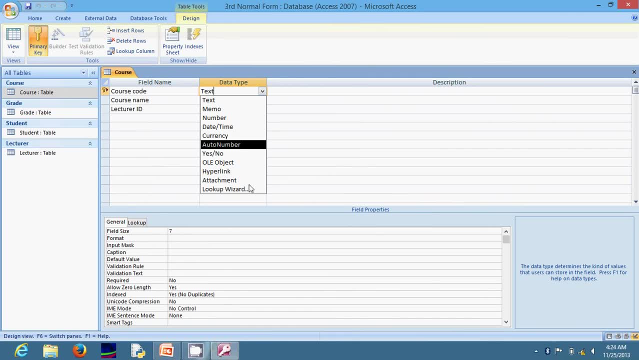 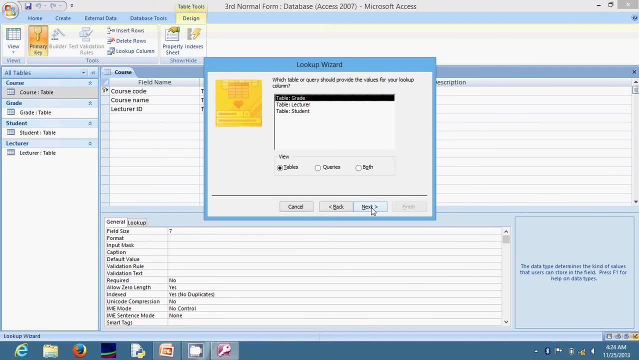 I'll go to course code Change this to lookup wizard. Of course, what I want to do is look up the column And is it from table? Yes, I'm doing that for table grade. Yes, So next My interest is in course code. 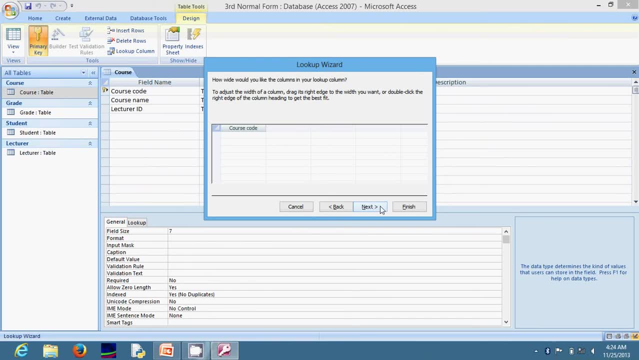 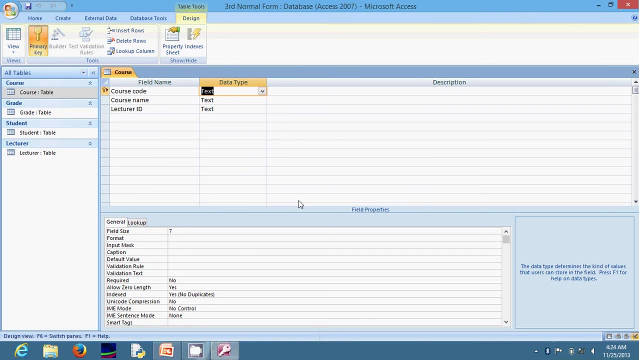 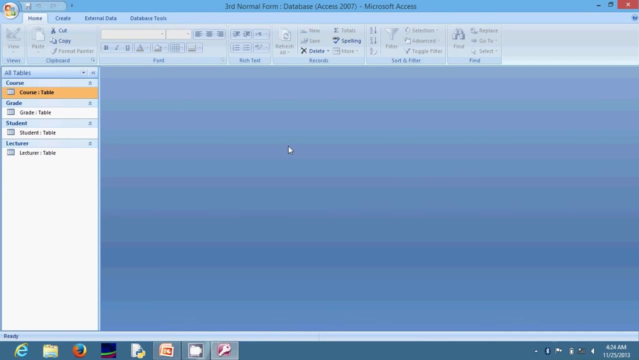 I transfer the course code to selected fields. Next, I'm okay with this And finish. Does it prompt me to save? Yes, Now, having done that, I can close this field. Now I do another lookup to link student matric number in table. 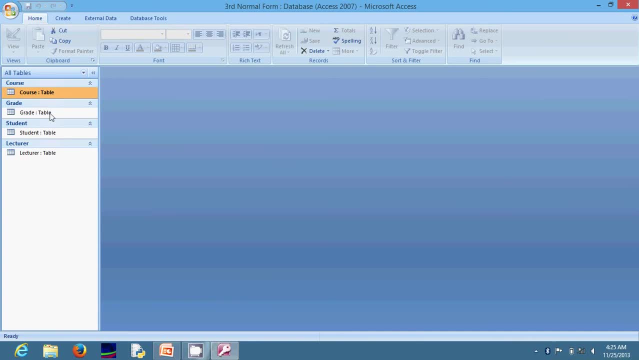 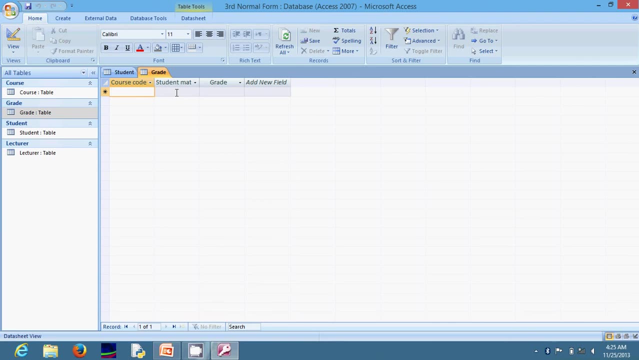 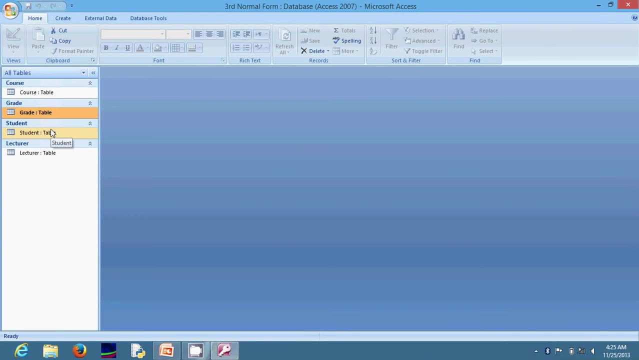 Yes, Student matric number in table: student to student matric number in this table, student to the student matric number I have in table grade. So let me quickly do that. So in this case, table grade is still my target. 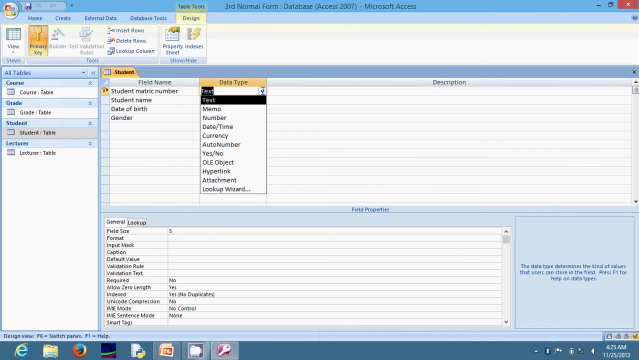 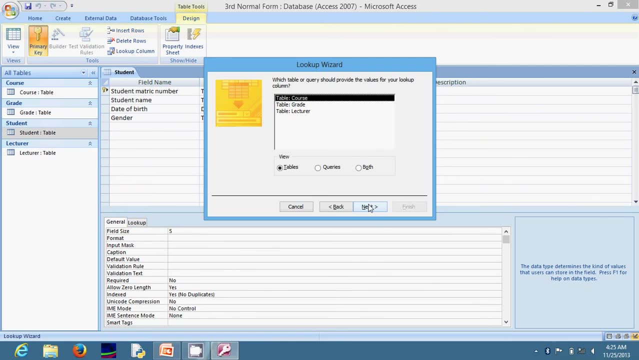 So I pick student Student matric number. I change this to lookup wizard, Of course. next Table grade is my target, So I change this to table grade And next Student matric number is my target. Next. 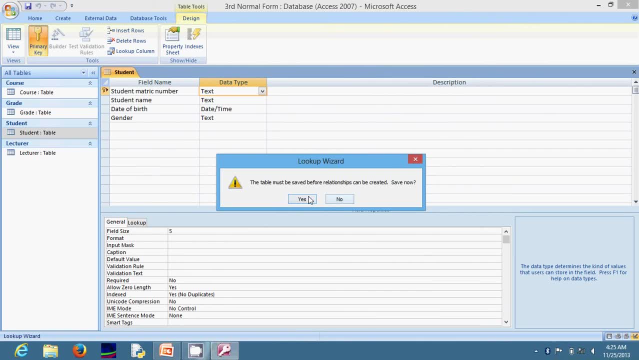 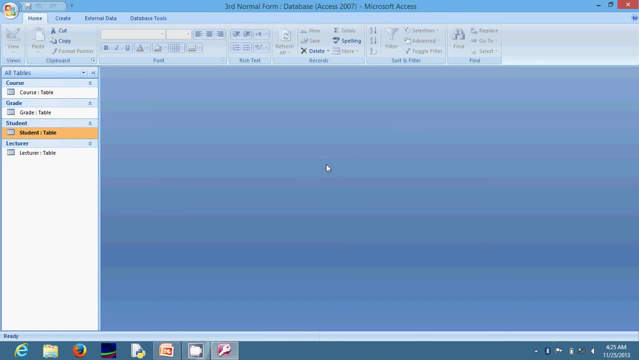 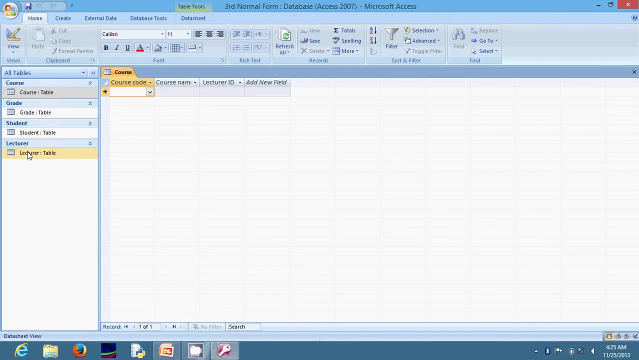 I'm okay with this And finish. Yes, Of course I want to save. Alright, Now, once you're through with that, you do one more lookup, And that last lookup is to link lecturer ID- Lecturer ID in this table course- to lecturer ID in this table- lecturer. 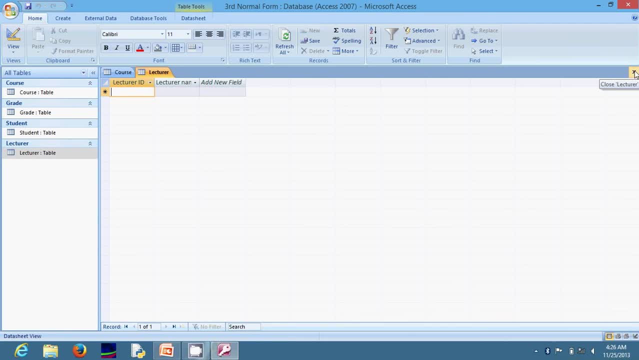 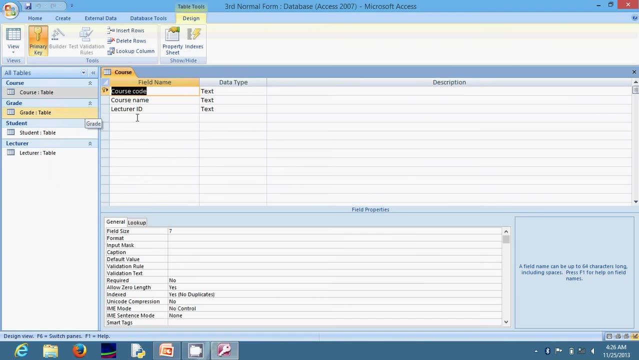 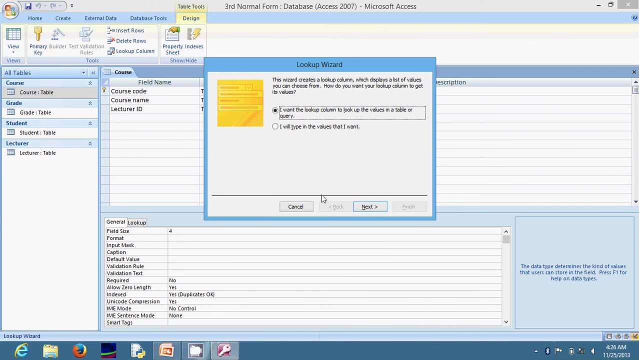 So in this case, table lecturer is my target. Table lecturer is my target, So I'll go to table course Design view Lecturer ID Lookup wizard. Next, Table lecturer is my target. Next, Lecturer ID is the field I'm interested in. 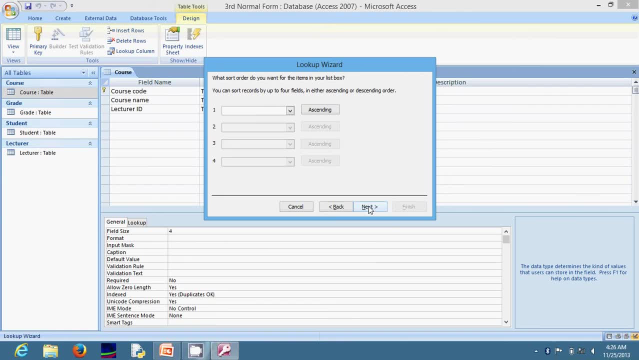 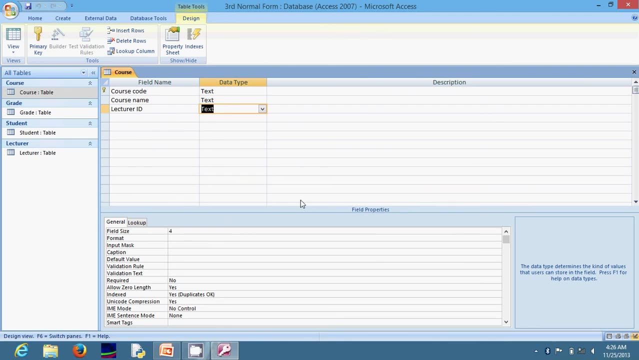 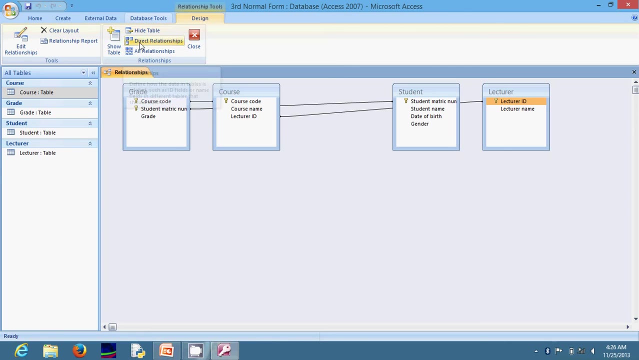 I transfer it to selected fields. Next, I'm okay with this. Next, Then finish And I will save Now. once you've done that, you can go ahead and check the relationships Database. to relationships: Now you can see a link between the table. 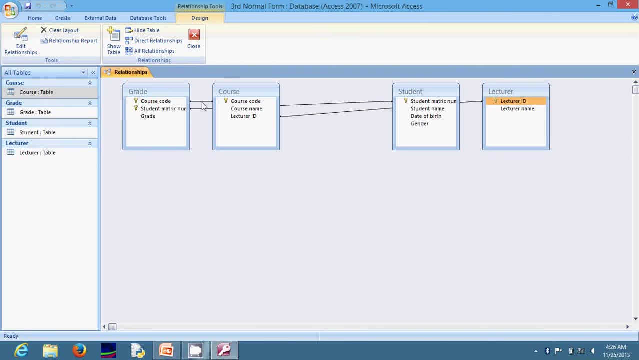 Now this table grade, table course. they are linked together with course code And table students and table grade linked together with student matrix number, Then table lecturer and table course linked together with lecturer ID. You can see that there is no table that is isolated. 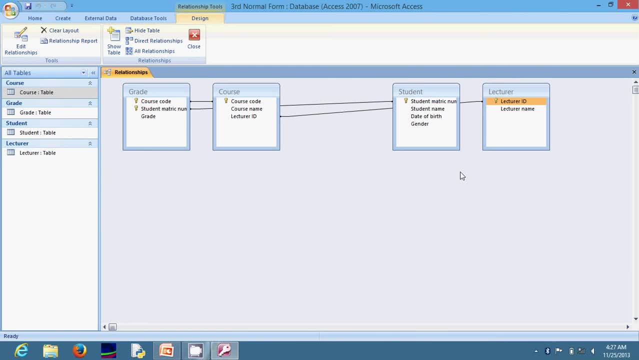 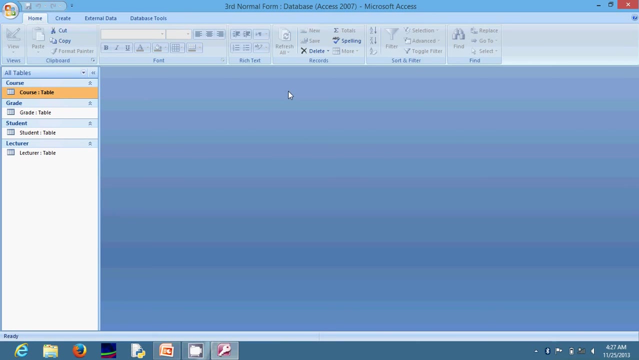 And that is the way your database should be. No table should be isolated. They should be linked together, And that's the essence of this connection. we're doing Alright, So we can close this, Alright. So the next thing we're going to do now is to populate our tables. 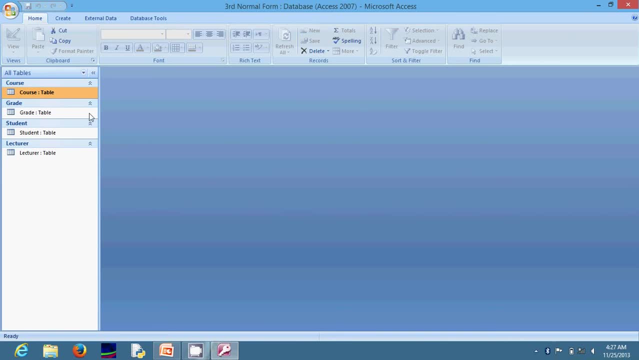 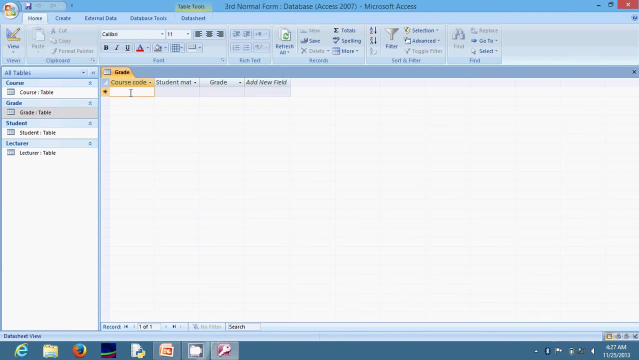 To populate our tables. I'm going to start with the target. Let me start with table grade For table grade, course code. You know we've been using different course codes. Let me use start with NTH101.. And the student matrix number I'll be using for this. 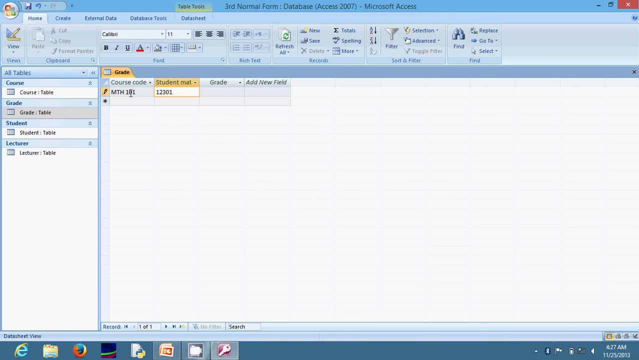 number I'll be using for this would be one, two, three, zero one. then I'm the grid. let's say the grid for this is A go for another one: CSC 101, the student matrix number. let me use the same matrix number and the grid for this would be P. let me do one more. 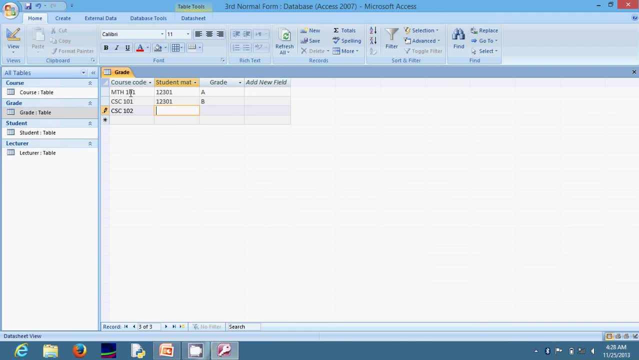 CSC 102 and the students I'll be using for this. I'll be using my coup when two, Three zero two and um for the name, let me use them. give you something. no for the grid. rather sorry for the grid to see, let me just see. all right, so i have. 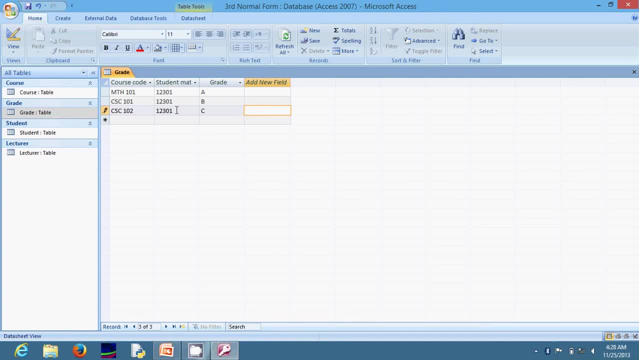 this. once i'm done with this, i can go ahead. no, no, no, i'm not using the same metric for this. let me just use one, three, two, three zero two. i think it's better this way. all right, so i can go ahead and save, then close this. so let me populate the next target, which is a lecturer table. so for this. 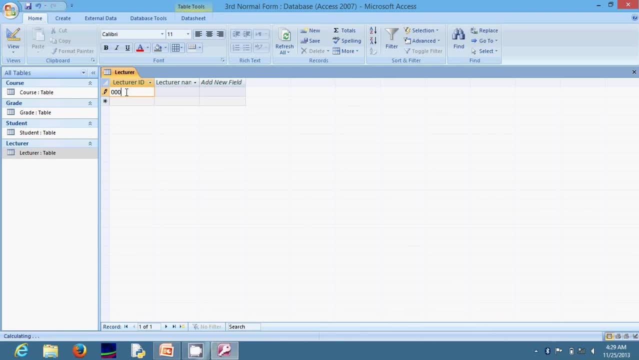 the lecturer id. let's say i have um zero zero zero one. the name of this man is smith, and i have another one zero, zero, zero two. let's say the name of this man is um. let me just stop with this string. i think it's cool. you can do as much as you like. um, let me save.